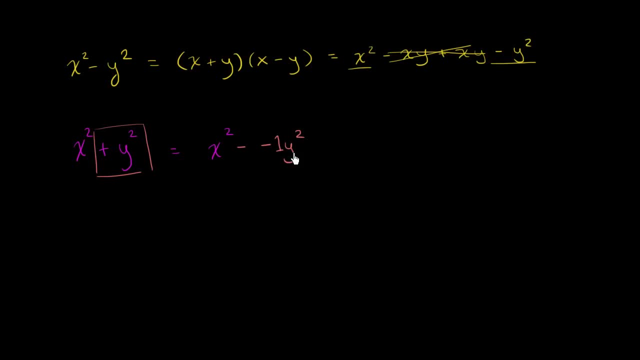 Well, this is the same thing as subtracting negative one times y squared. Now, what is if we wanted to write this whole thing as a square? if we wanted to rewrite, if we wanted to write this whole thing as a square, how would we do it? 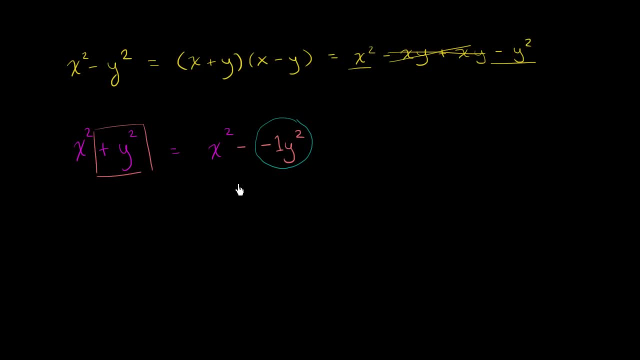 Well, we have y squared. and what's negative one? the square of? Well, we know, by definition, negative one. by definition, negative one is equal to i squared, or that i is equal to, or i squared is equal to negative one. 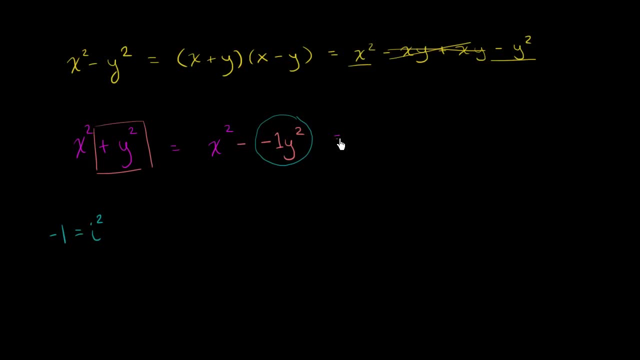 So let's rewrite it that way. So this is going to be equal to x squared minus instead of negative one. I'll write that as i squared minus i squared y squared. All I replace, all I do, is I replace this negative one with an i squared. 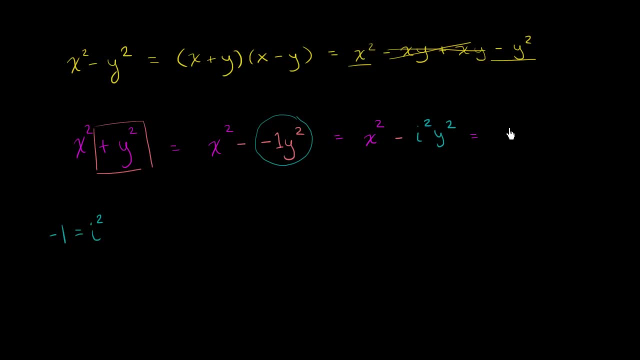 And now this is interesting. I think you see where this is going, but I'll just make it very explicit. This is now x squared minus x squared minus minus i, y squared. And just like that, using i, I've been able to write this sum of squares. 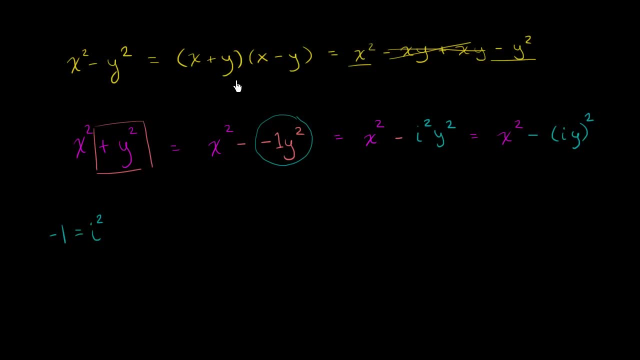 as a difference of squares. And now we can factor it just the exact same way that we factored this original expression: This thing is going to be equal to. so it's going to be equal to x, x plus this thing: i y. 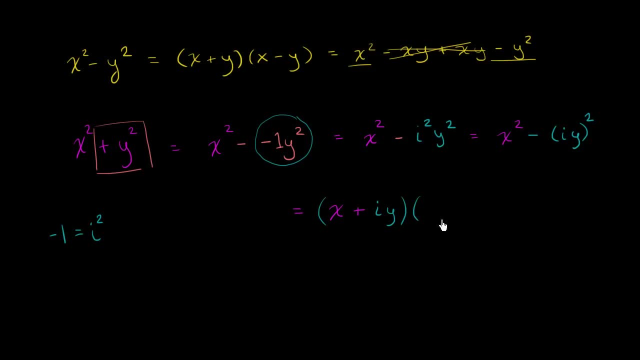 x plus i y times times x x minus i y, x minus i y. And we can verify that. if you multiply these two expressions together, you're going to get x squared plus y squared. Let's do that. Let's do that. 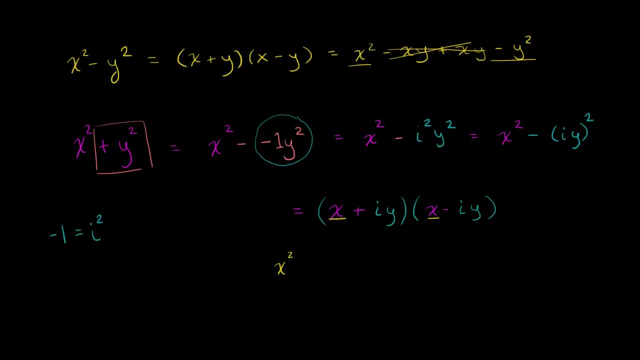 x times x is x squared, x times negative. i y is negative. i x y. And then i y times x. i times x is positive: i x y. And then finally, finally, let me do this in a color I'm not using yet.